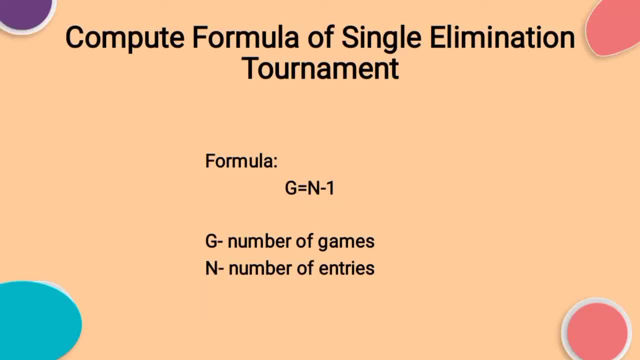 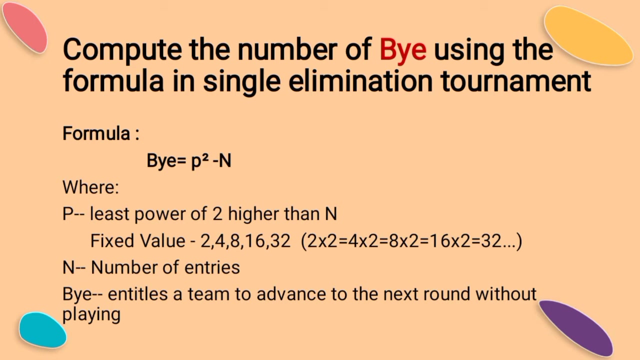 elimination tournament. so we have here: G is equals to n minus 1, so G refers to the number of games and n refers to the number of entries. so now let's proceed to the by. so how to compute the number of? by using the formula in single elimination tournament. so this is the formula: by equals p squared minus. 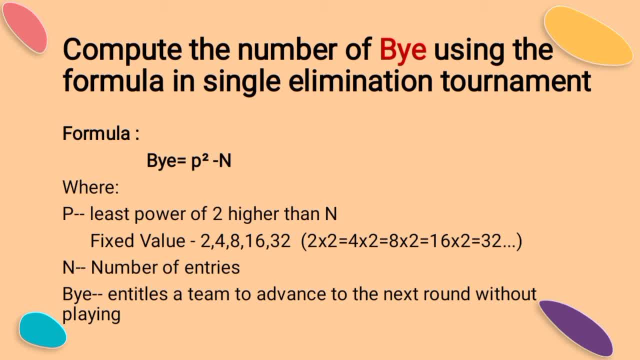 n. we're P less power of 2 higher than N. so these are the fixed value: 2, 4, 8, 16, 32 and so on and so forth. or 2 times 2 is equals to 4 times 2 equals 8 times 2. 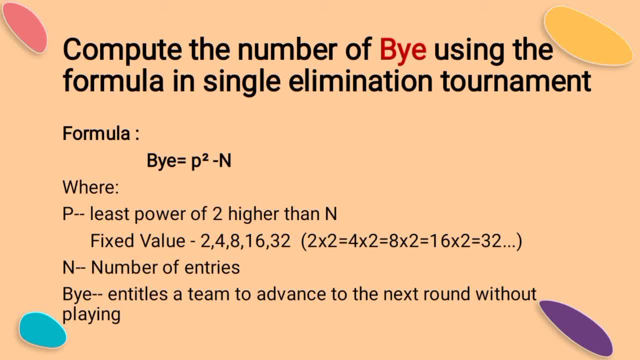 equals 16 times 2 equals 10.. two equals to 32, and so on and so forth. so n is the number of entries by the entitles a team to advance to the next round without playing. so, for example, if team one is a buy, so he will directly. 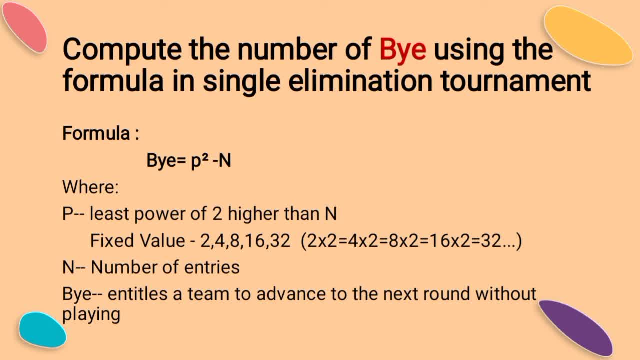 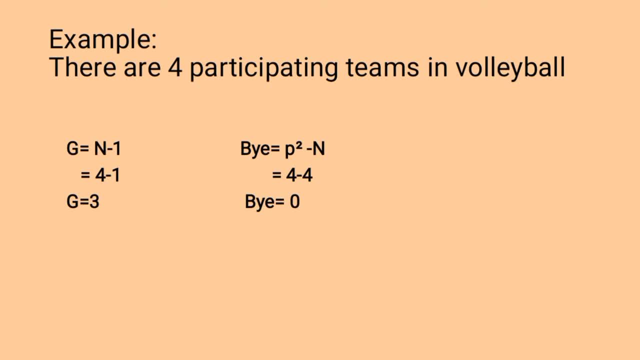 advance the next round without playing the first round. so, for example, there are four participating teams in volleyball. so the formula of games is: g equals n minus one. then four refers to the teams. four teams minus one is equals to three. so we have in four teams. we have 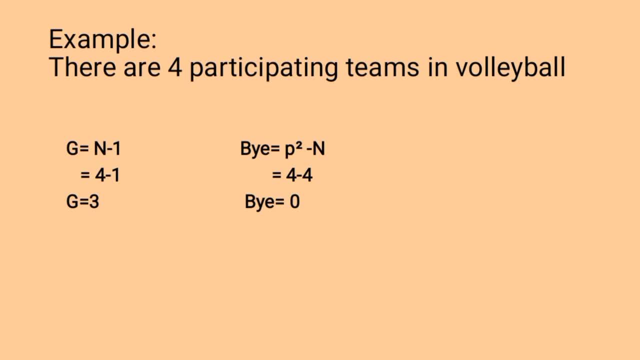 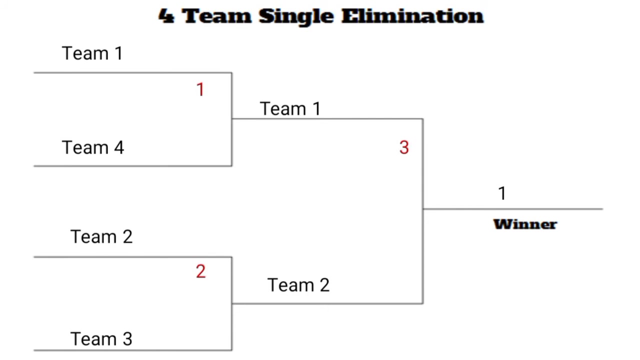 three games. then for the buy buy equals p squared minus n, then four, four- here is the fixed value- minus four the participating teams. so four minus four is equals to zero. so we have no buy in um four teams and lastly, we have teams single elimination. so this is the bracket and the illustration of how the game is being.